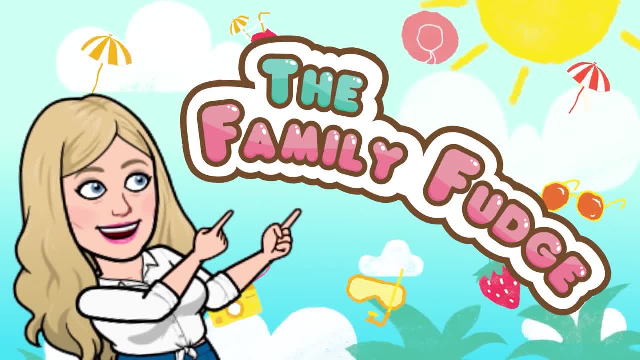 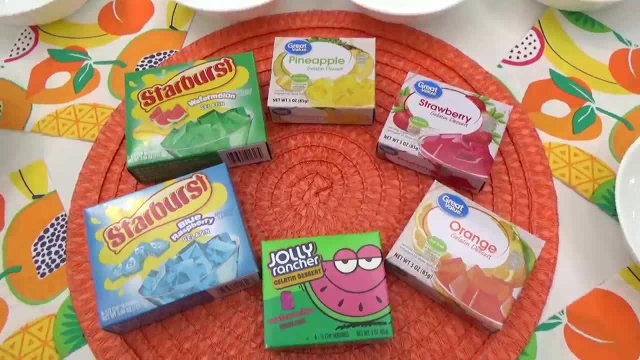 Hey guys, Jennifer here and welcome to The Family Fudge. In today's video, my kids and I are headed into the kitchen to whip up four quick and easy no-bake treats. These treats come together so quickly. They only require a few ingredients. 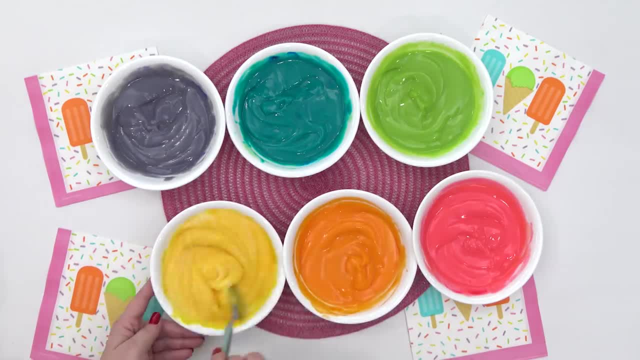 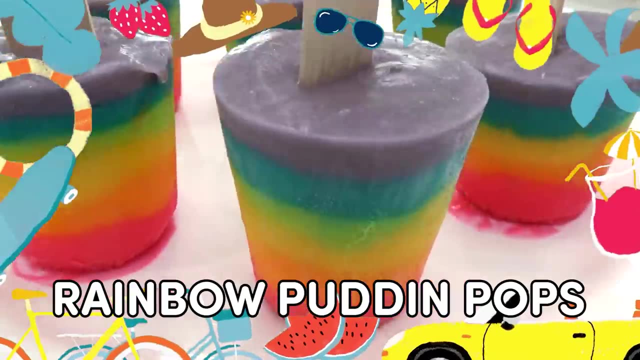 and the best part is, since these desserts are no-bake, they are perfect for little kids to help make or for bigger kids or teens to make for themselves. In today's video, I'm making rainbow pudding pops, watermelon rice crispy treats. 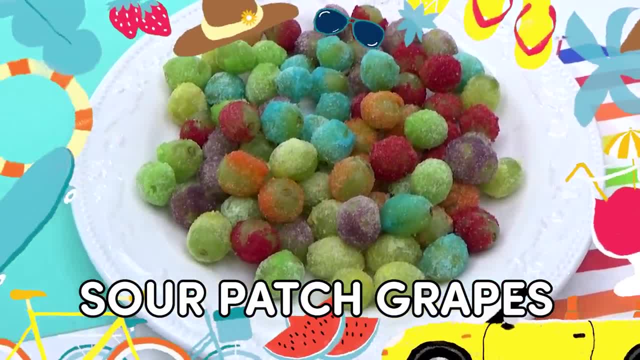 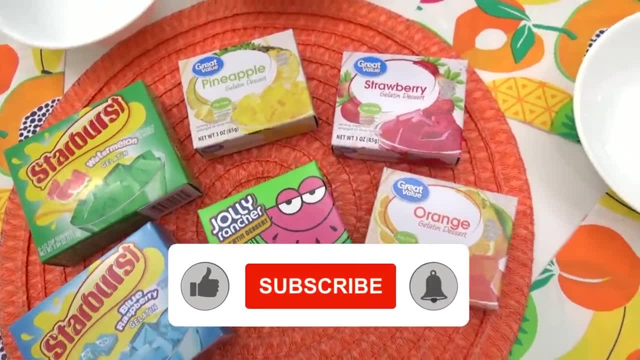 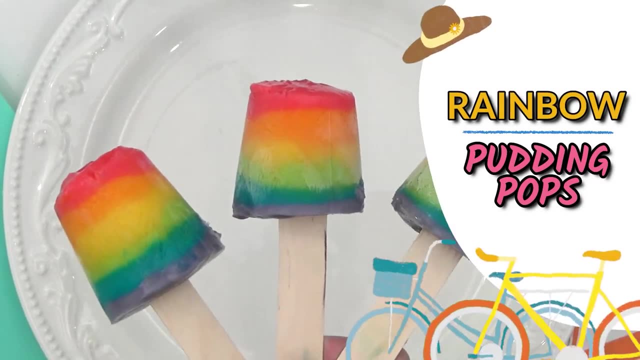 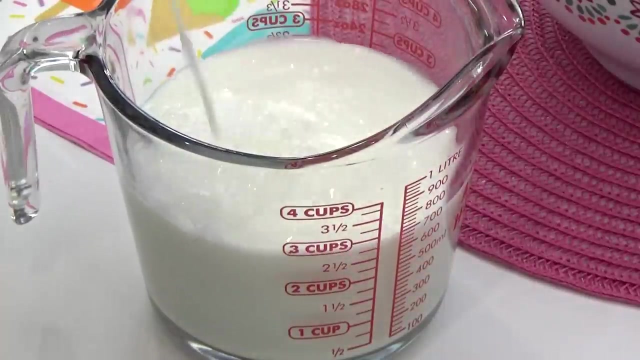 the TikTok famous Sour Patch Grapes and my favorite blueberry bagel bites. Now I'm kicking things off with a super cool, creamy and colorful treat. For this recipe, we're going to start by adding six cups of milk to a large mixing bowl. 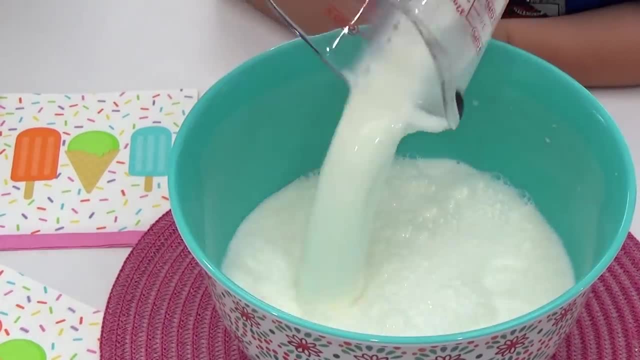 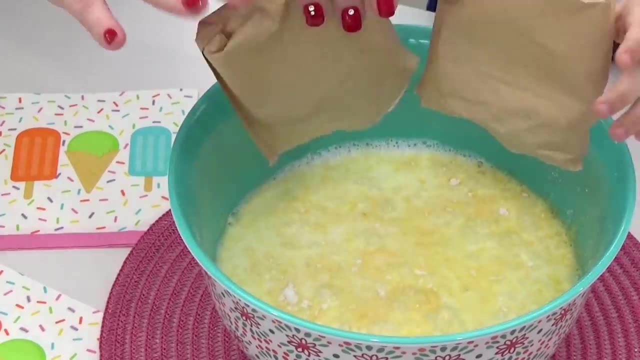 To this. Griffin and I are going to pour two boxes of instant vanilla pudding mix. And you guys, these are the bigger boxes of pudding mix, Don't get the small ones. Now, using our electric hand mixer, we're going to print bowls. 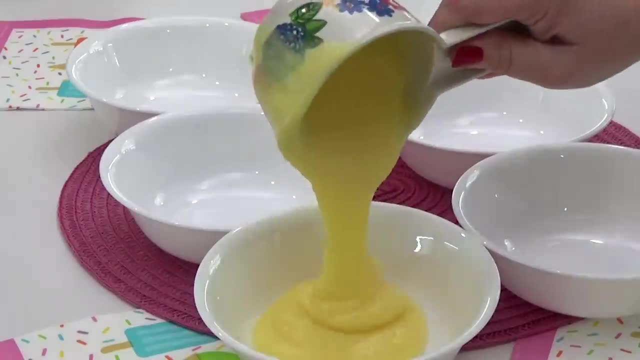 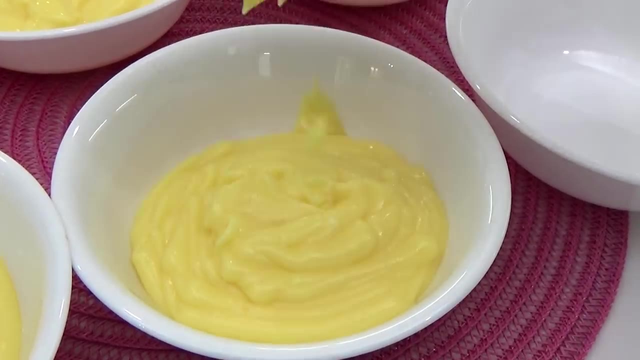 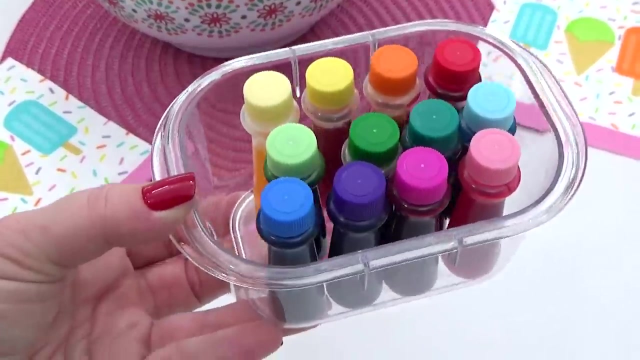 And you guys, each bowl is going to get around one cup of this pudding mixture. Now, to make these into rainbow pudding pops, I am going to add just a little bit of food coloring to each bowl And of course, the more food coloring you add, 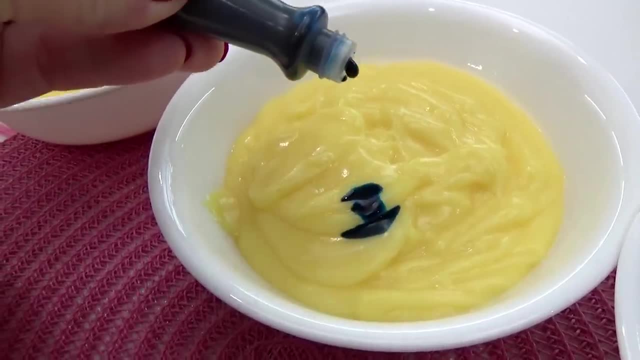 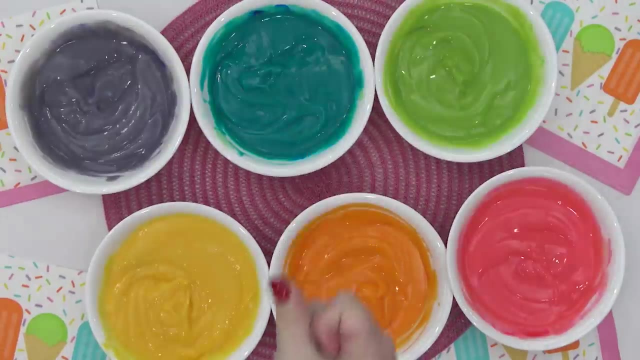 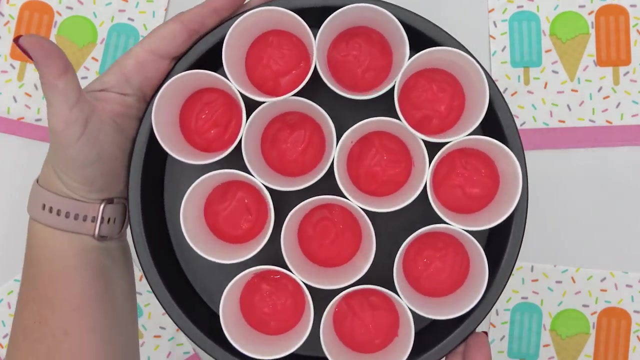 the more vibrant your rainbow will be. After we have all of these mixed together, it's time to spoon the pudding mix into these tiny paper cups. And you guys? I went ahead and added my cups to a baking pan like this. That way, it's going to be a lot easier. 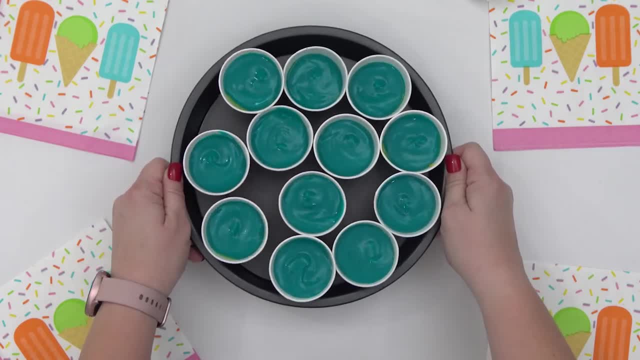 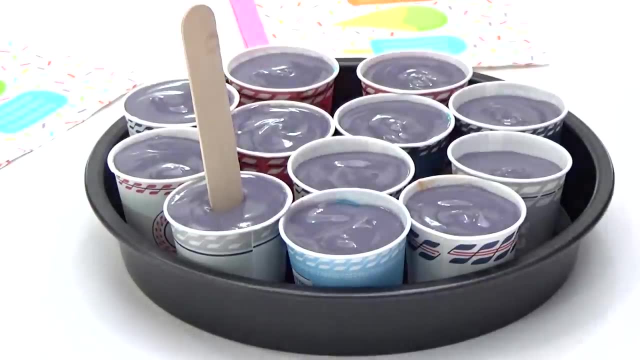 for me to transfer them to the freezer after they're filled. Now, you guys, these are pretty full, So now all I have to do is stick some popsicle sticks into each little cup. Then I'm going to stick the entire thing into the freezer. 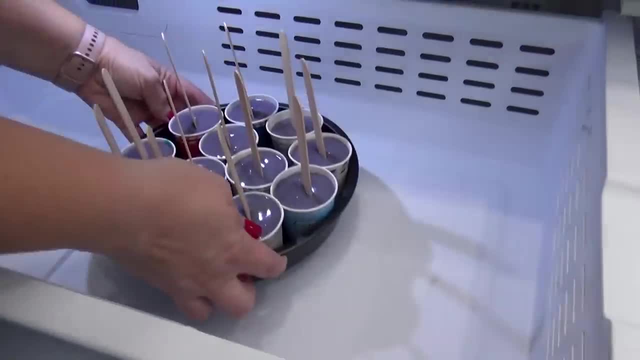 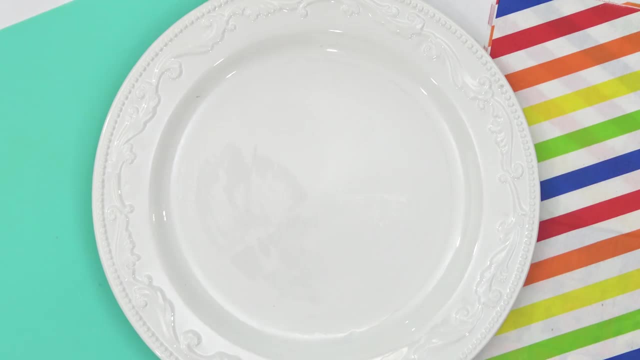 And you're going to want to freeze these for at least four to five hours, But if you can freeze these overnight, that would be even better. When you're ready to enjoy these pudding pop, all you have to do is peel off a little paper cup. 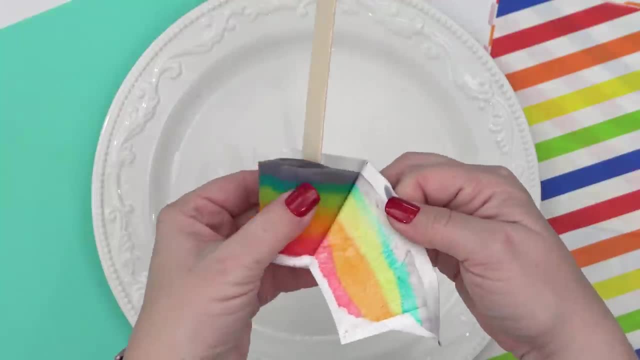 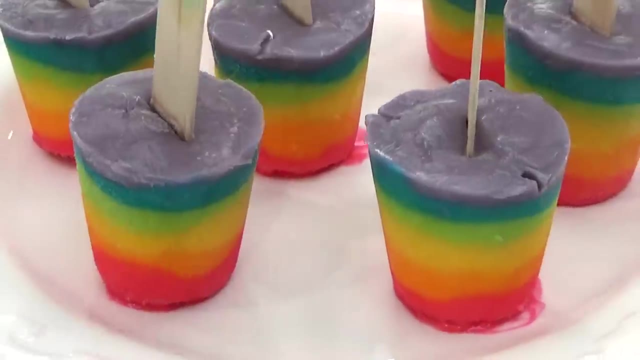 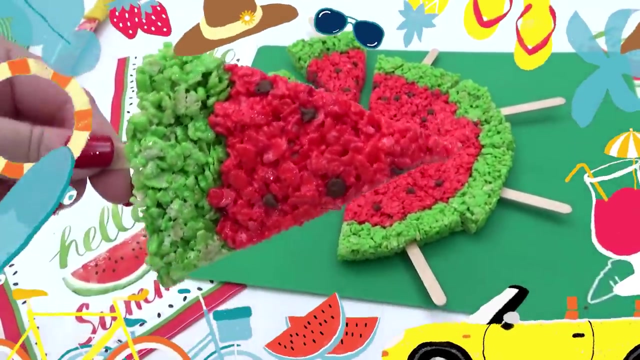 and you're ready to dig in. But just be warned: these do melt super fast on a hot summer day. Okay, guys, next up is a summer twist on one of our favorite no-bake treats. This recipe starts off with your typical Rice Krispie Treat ingredients. 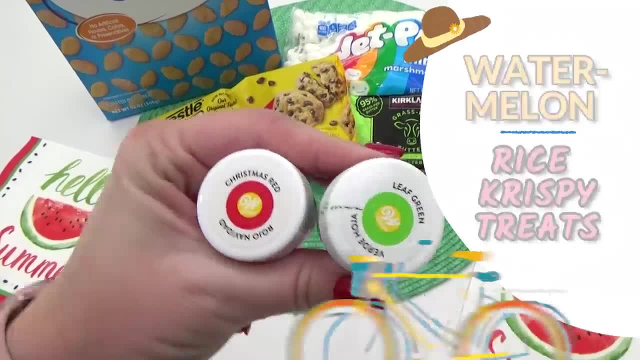 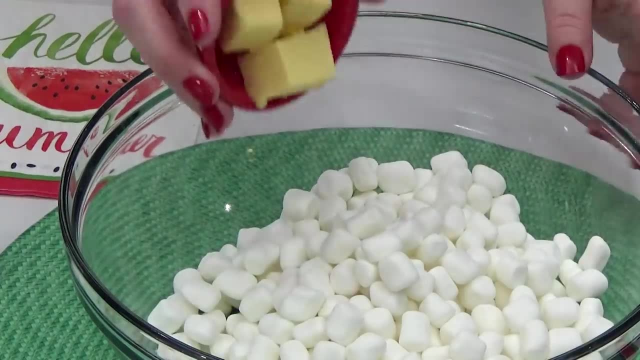 but there are a few fun extras. Now to get started, I'm going to take a large, microwave-safe mixing bowl and with this I'm going to add four cups of mini marshmallows, followed by three tablespoons of butter. Now I'm going to pop this into the microwave. 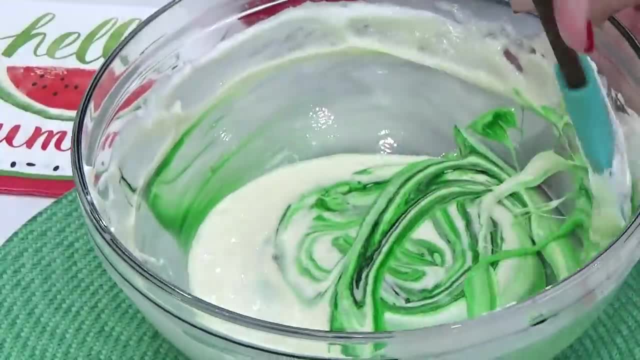 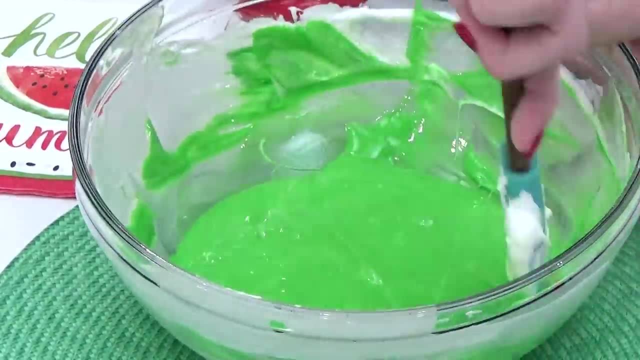 Once it's melted, I go ahead and add in the food coloring, And for this batch I'm adding green, because I want this to kind of look like the rind of a watermelon. Once I have that all mixed together, it's time for this cereal. 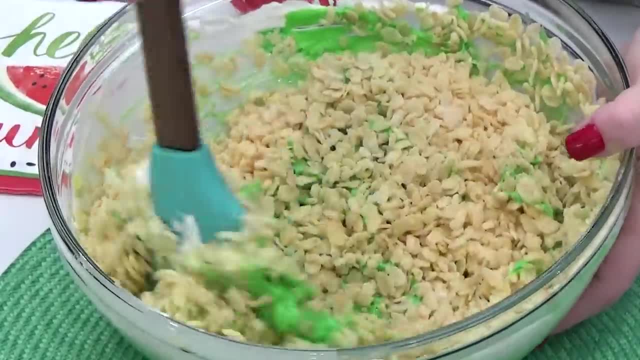 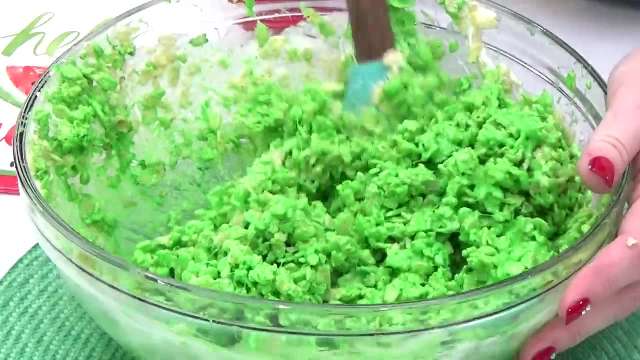 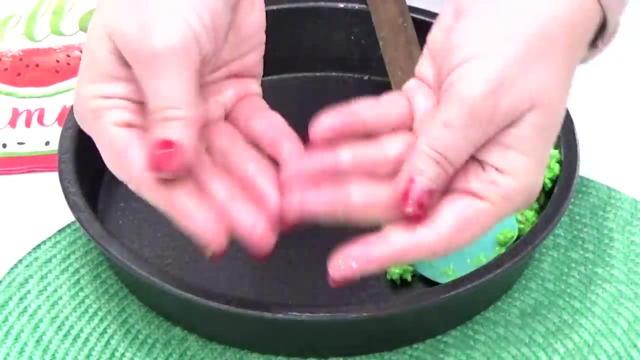 I'm adding four cups of Rice Krispie cereal, and then I'm going to use my muscles to get this all stirred together. Just mix this in the microwave for about a minute and then add the sugar. Once that step is done, I'm going to add half of this mixture. 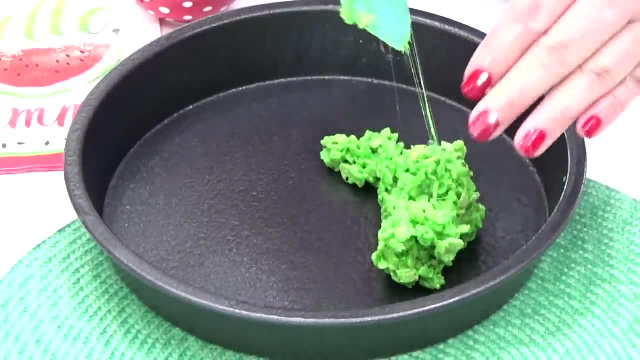 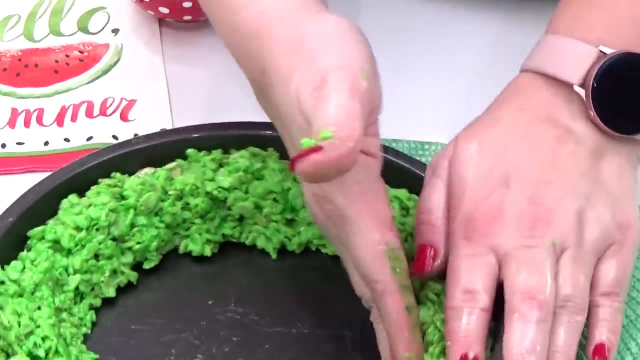 into each of my two round cake pans, which I've already sprayed with nonstick spray. Then you guys, using my well-greased hands, I'm just going to mold this all around the edges of the pan, and you wanna make sure to leave a spot open in the center. 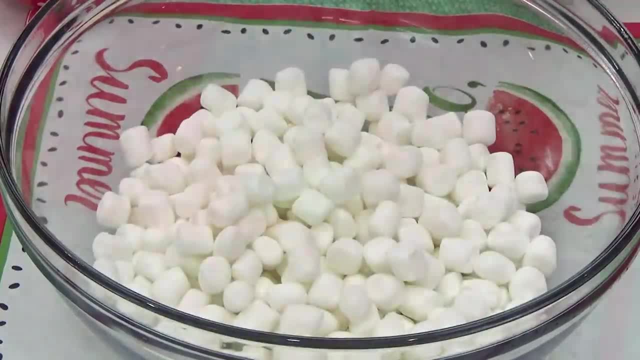 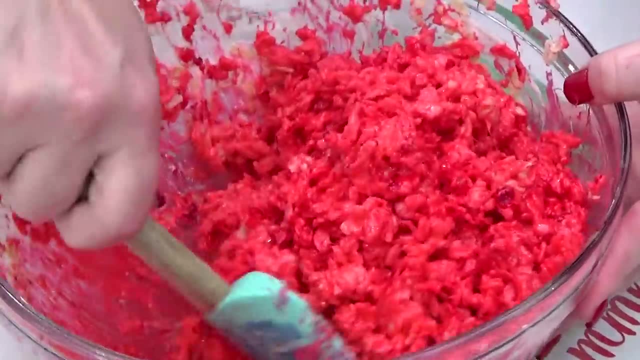 for what's to come. Next up is the red batch, which starts just the same way as the green batch. Again, I'm adding four cup of mini marshmallows and three tablespoons of butter. Half this will go in one pan and half will go in the other. 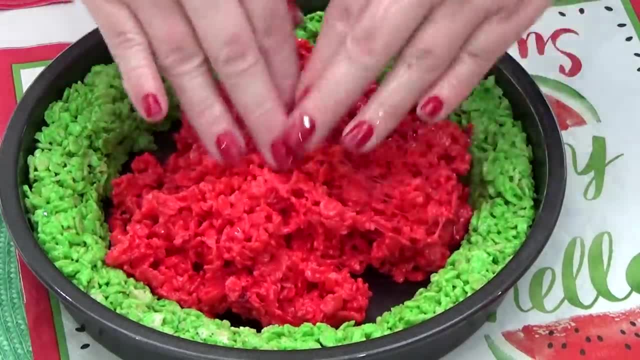 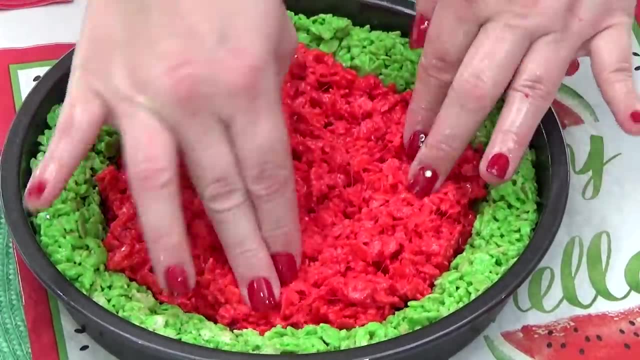 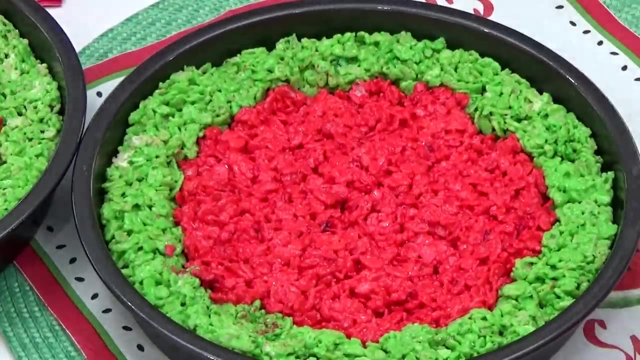 And you guys. at this point I'm going to really press this together super well, especially at the seams where the two colors meet. I really wanna make sure that the two colors will end up sticking together. And now, you guys, to finish this off. 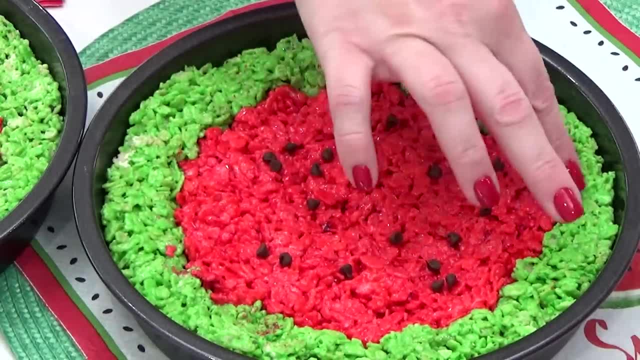 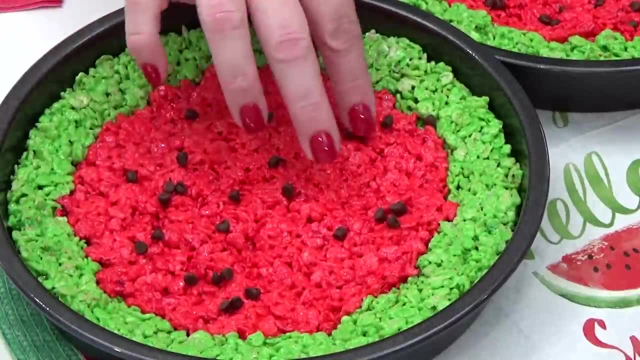 I'm just gonna be sprinkling a few mini chocolate chips right on the top And that's to kind of look like the seeds of the watermelon, And I am going to kind of gently press these into the top just to make sure that they don't fall off. 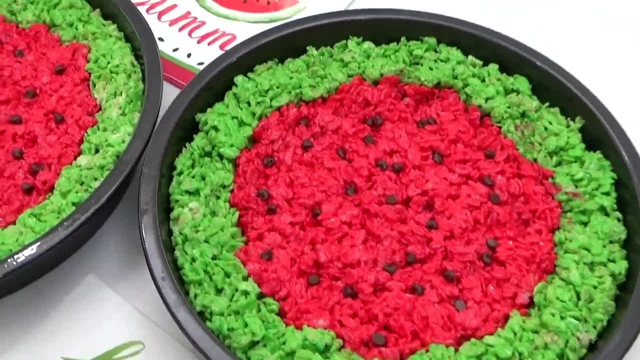 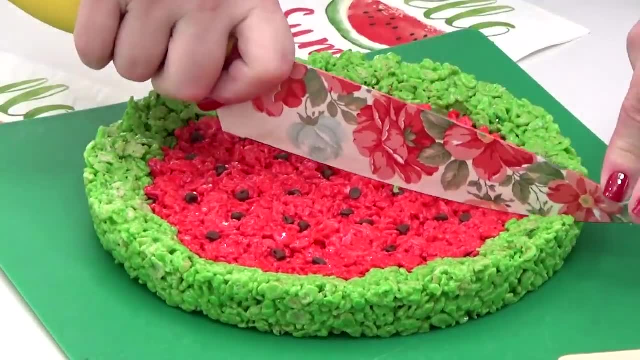 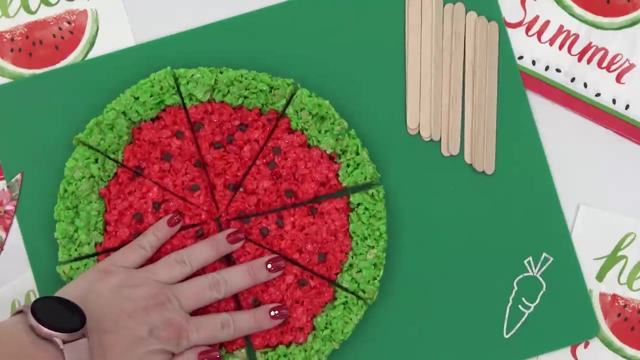 Now I'm going to set these aside for about an hour or so, or until they're hardened enough to cut into them. And you guys, to make it even more fun and super portable, I'm just gonna go ahead and add one popsicle stick. 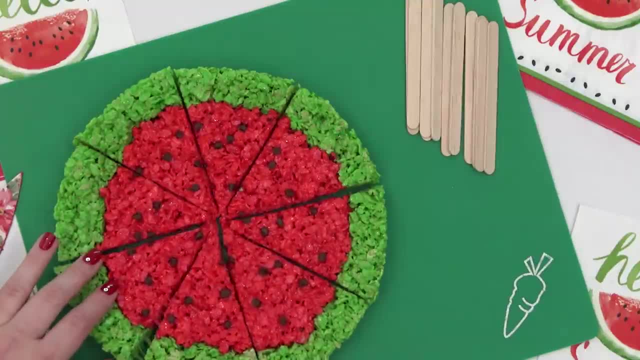 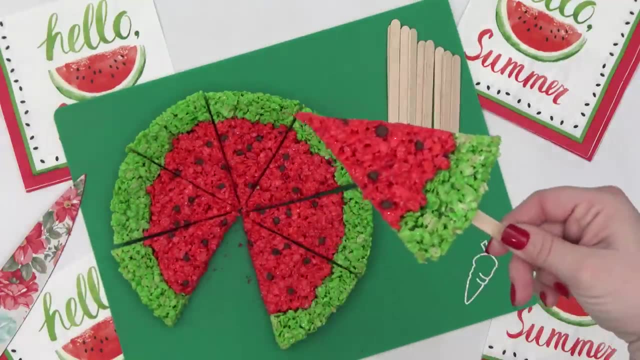 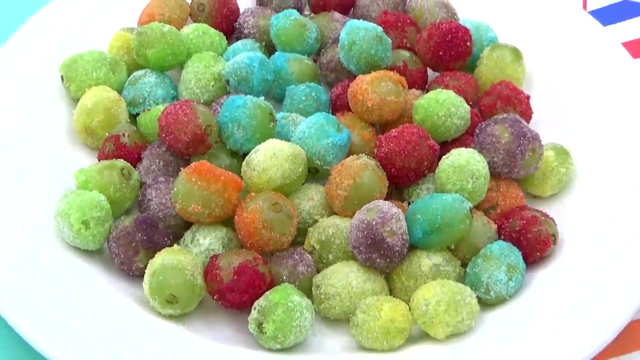 into each of the watermelon wedges. Now, you guys, these were seriously so quick and easy to throw together. Of course, they taste delicious And I really think these turned out super cute. Okay, guys, now that brings me to a new sweet. 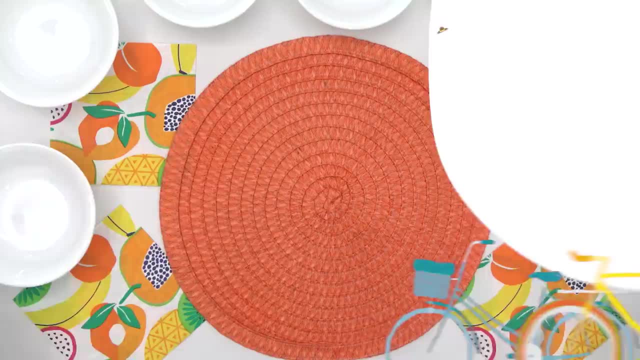 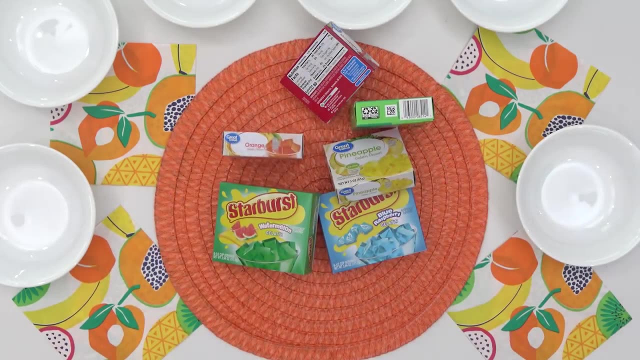 and tangy treat that I learned about on TikTok. For this, all you're going to need are grapes and Jell-O. Now, of course, you can use whatever flavor of Jell-O that you prefer. Since I love rainbows, I'm gonna go ahead. 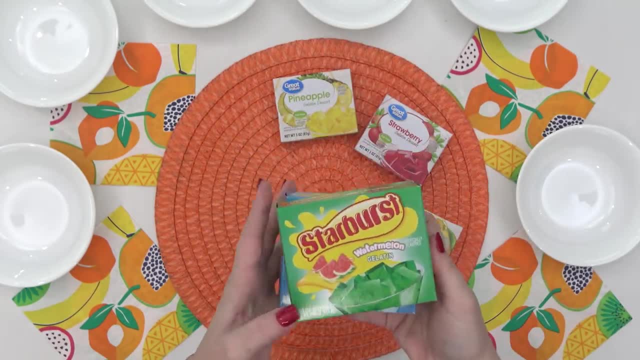 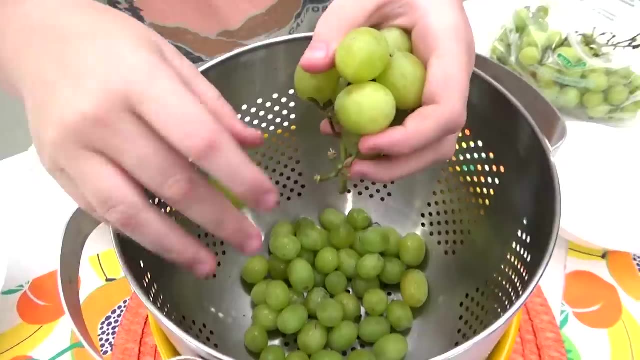 and use six different colors and flavors of Jell-O. So now McKenzie and I are going to start by taking the grape off of the stem, Then we're going to take them over to the sink and give them a good whopper. Okay, so now we're gonna take the grape off of the stem, Then we're going to take them over to the sink and give them a good whopper. 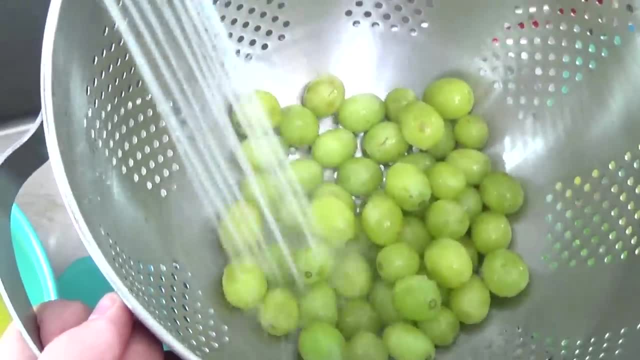 So now McKenzie and I are going to start by taking the grape off of the stem. So now McKenzie and I are going to start by taking the grape off of the stem. Next, I'm going to set up our little assembly line area. 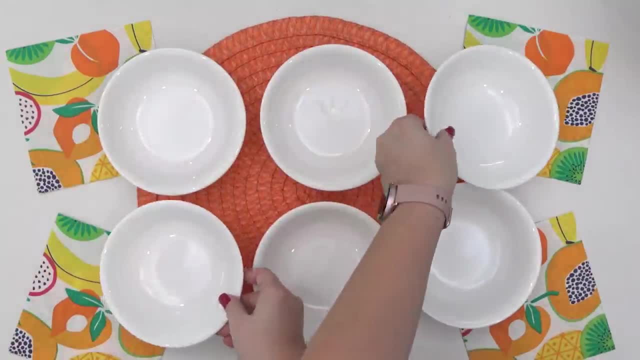 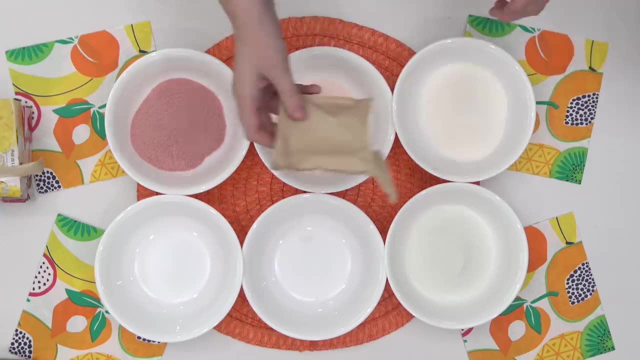 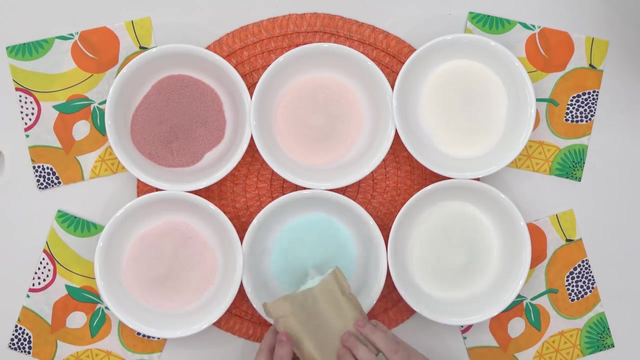 I've gotten out one bowl for each of the Jell-O flavors, and McKenzie and I are going to add the powder in to each bowl just like this. I also have plenty of toothpicks ready to go and a cup of water. 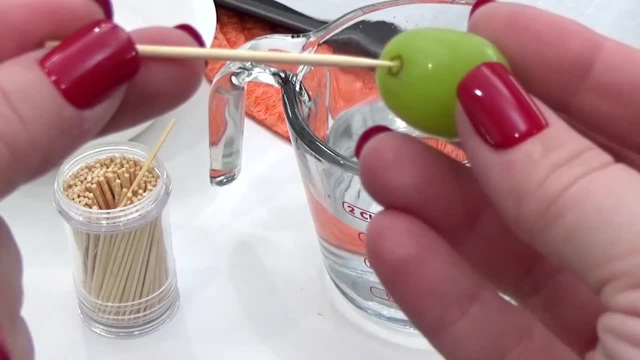 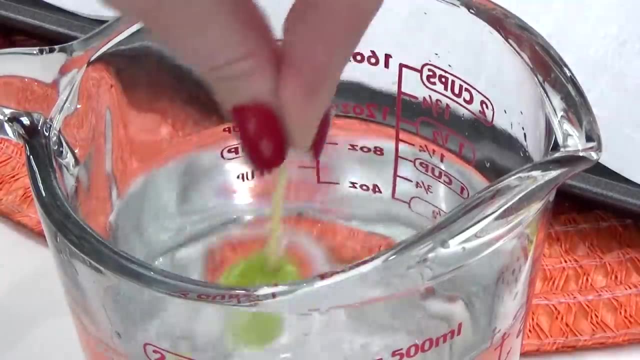 Now, basically, all you have to do is is add one grape at a time to a toothpick. Next you're going to dip that grape into some water, then quickly roll the grape in the Jell-O powder, just like this. 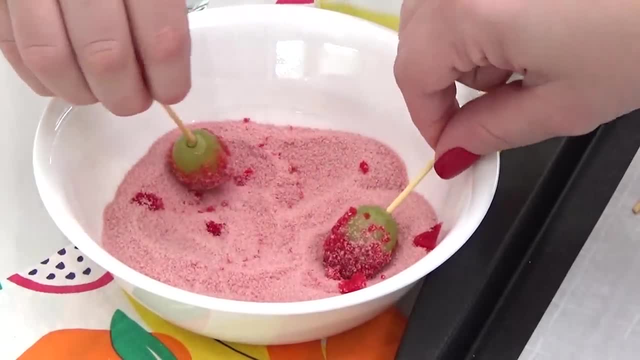 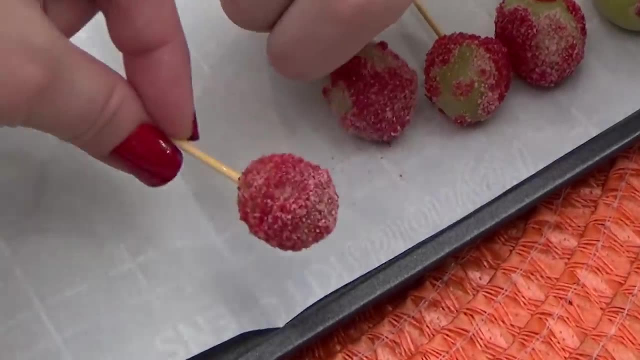 Now, sometimes the Jell-O sticks really well and sometimes it doesn't, but that's okay. Of course, the more powder you add, the sweeter your grape is going to be. So I actually prefer a thin coating of the Jell-O. 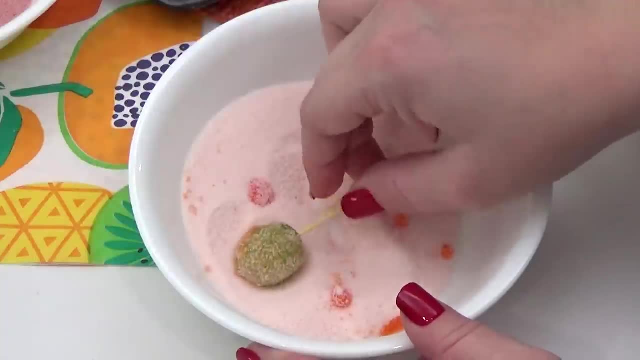 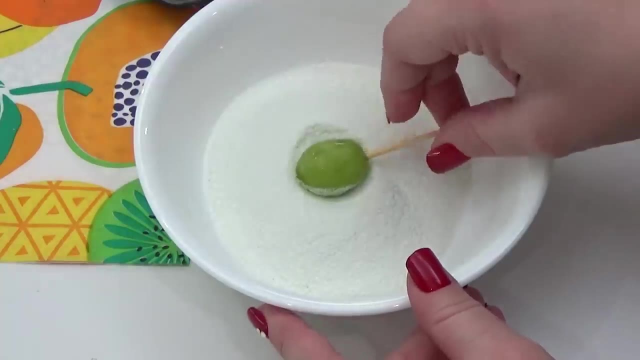 Now, as these dry, the Jell-O is gonna become kind of like a crunchy shell on the exterior of the grape, And with the combination of the sweet and the sour, these grapes really do taste a lot like Sour Patch Kid candy. 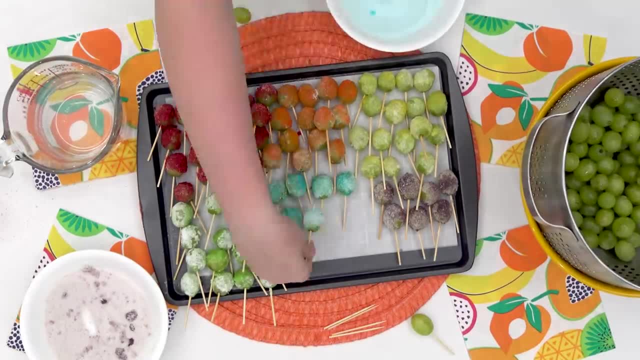 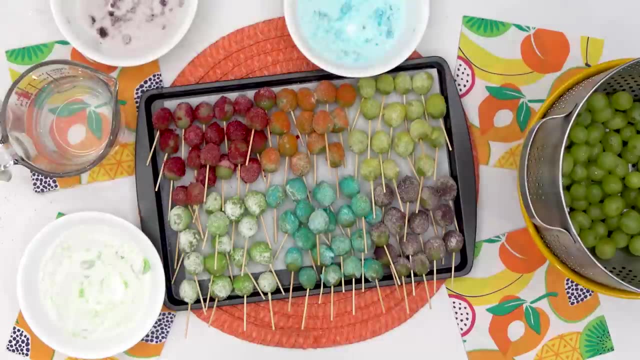 Once you have all of your grapes dipped, you're just going to stick them in the fridge for about an hour so that the Jell-O can combine with the Jell-O and completely harden. And check these out, you guys. These came out so pretty. 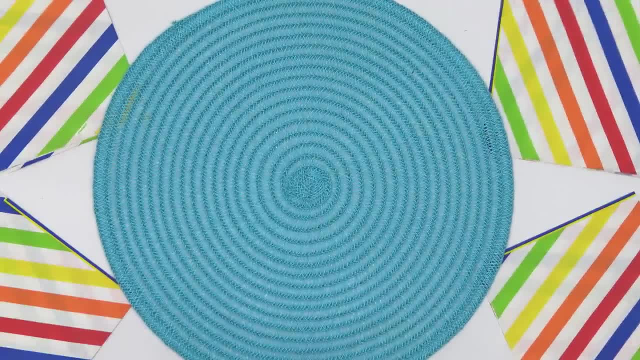 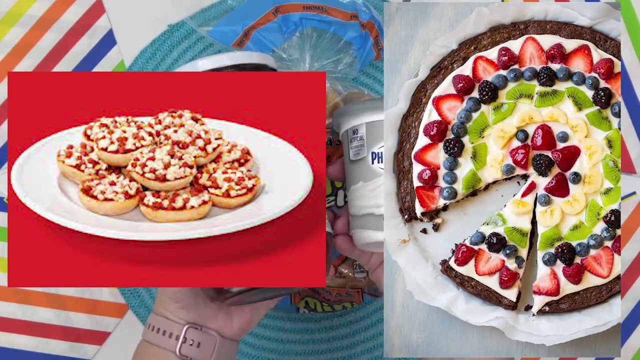 They almost look like little edible pebbles. Okay, guys, now that brings me to a treat that's kind of like a cross between a bagel bite and a fruit pizza. For this, we're going to be using some mini blueberry bagels. 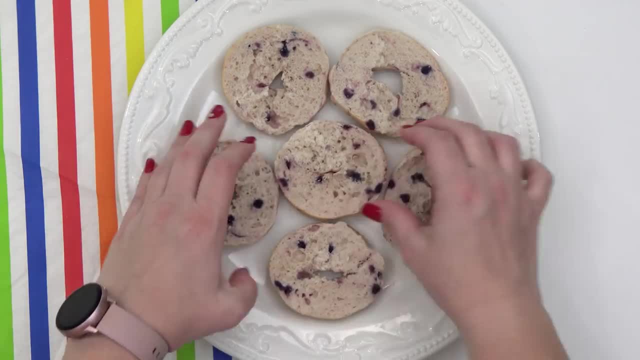 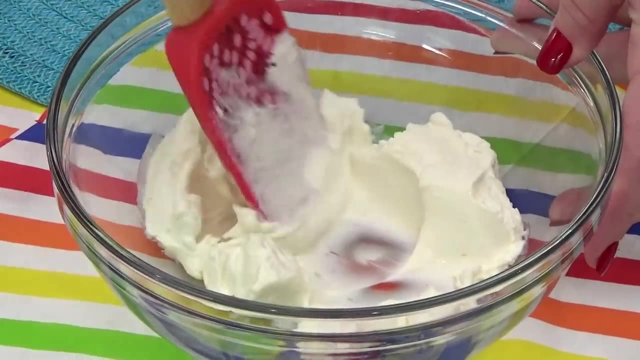 and I'm gonna go ahead and split them apart just like this. That way they're ready to go. And now I'm gonna go ahead and make the delicious sauce. And you guys, for this, I'm just gonna be taking two simple ingredients: some plain cream cheese. 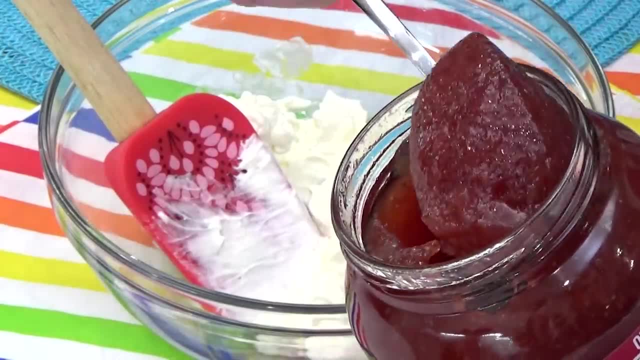 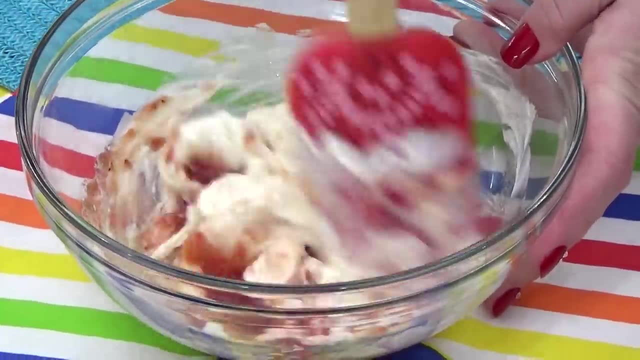 this is room temperature and some jam. Now, of course, you can use whatever flavor jam you like, but I really like to use strawberry jam for this, because when the strawberry flavor mixes with the cream cheese, it almost tastes like a strawberry cheesecake filling. 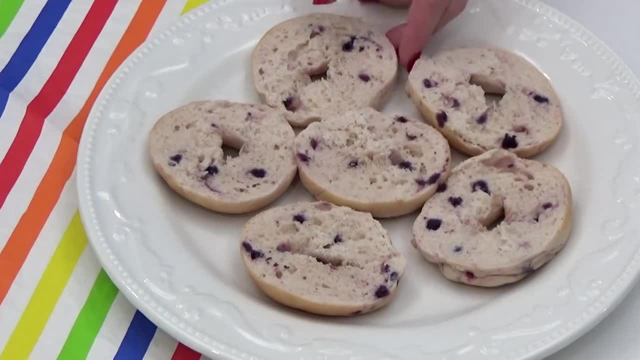 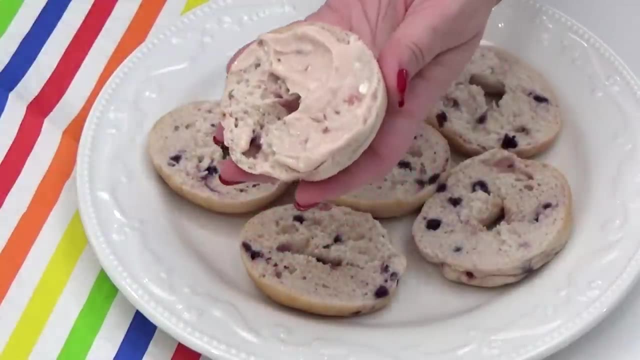 So now that I have this all mixed together, I'm gonna go ahead and spread a good amount onto each bagel And, of course, if you wanted to, you could toast the bagels before this step, but in our house really prefer a softer bagel. 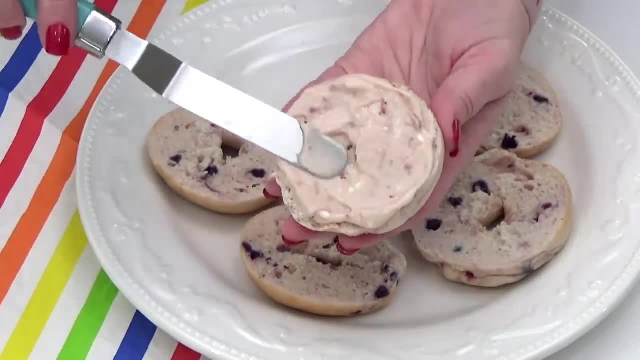 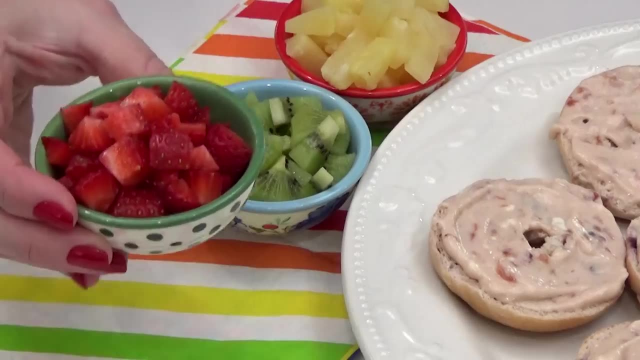 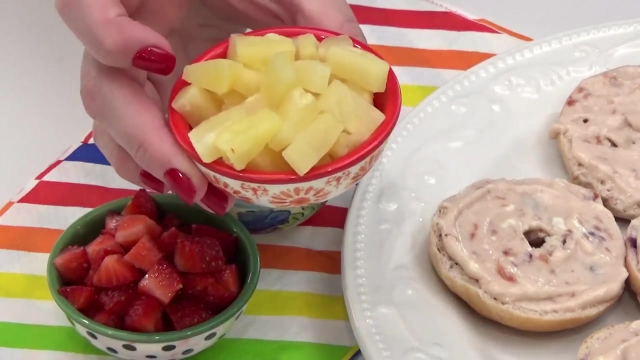 though I didn't toast these at all. So once the cream cheese is on there, it's time for the toppings, And in this case, instead of pepperoni and cheese and olives, we're using fresh fruit, And in this case, instead of adding. 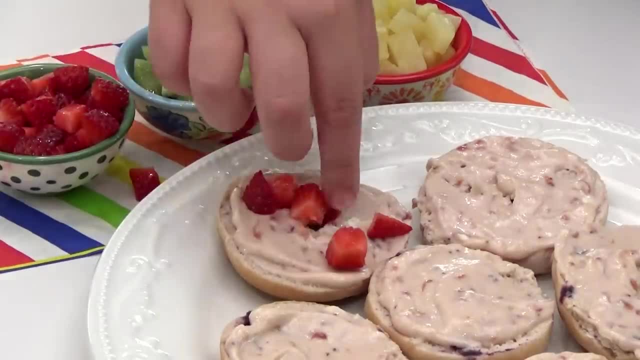 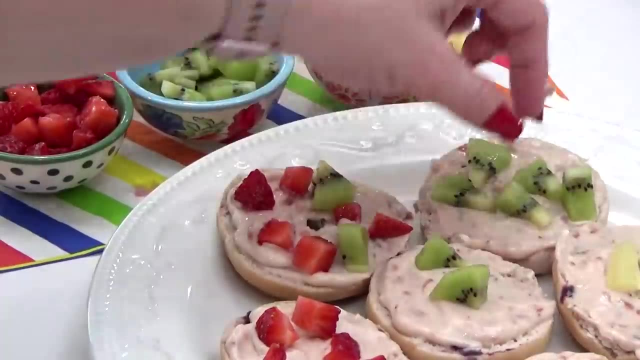 and in this case, for these pizzas, we're not using pepperoni or sausage or olives, but instead Jackson and I are gonna be adding lots of fresh fruit that I cut into really small pieces. We have some strawberry, some kiwi and some pineapple.